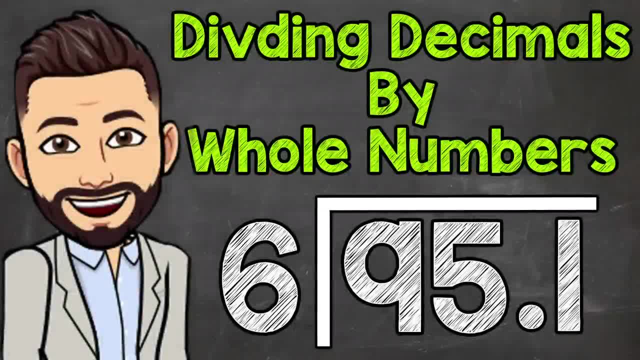 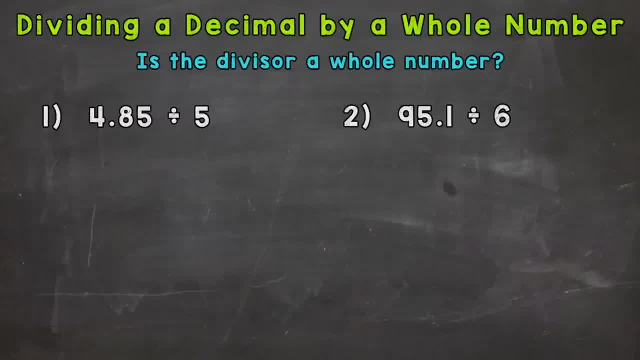 Welcome to math with Mr J. In this video, I'm going to be covering how to divide a decimal by a whole number. So we have two examples here that we're going to go through together in order to get this down. So let's jump into number one, where we have 4 and 85 hundredths divided by 5.. And the first thing we need to do is set this problem up. So 4 and 85 hundredths here, this is our dividend, It's the number that's. 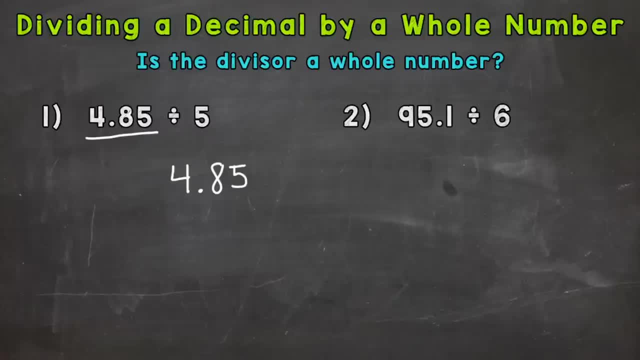 being divided or split up. That goes underneath the division bar And we are dividing by 5. So 5 is our divisor. It goes on the outside. Now, once we have our problem set up, whenever you see decimals within a division problem, you need to ask yourself a question, And it's at the top of 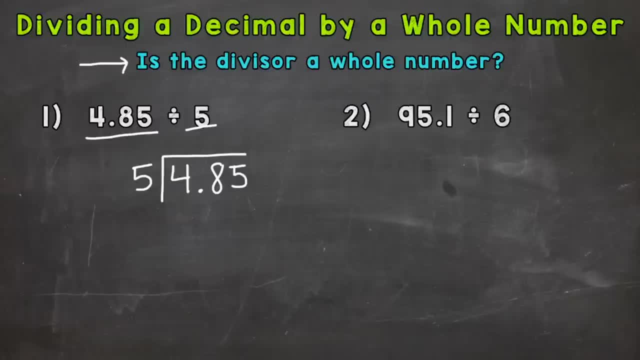 your screen. Is the divisor a whole number? And if so, if your divisor is whole, you can bring your decimal straight up. That's where it's going to go in the answer And in the case of this video, our divisors are going to be whole, So we can bring that decimal straight up Once. 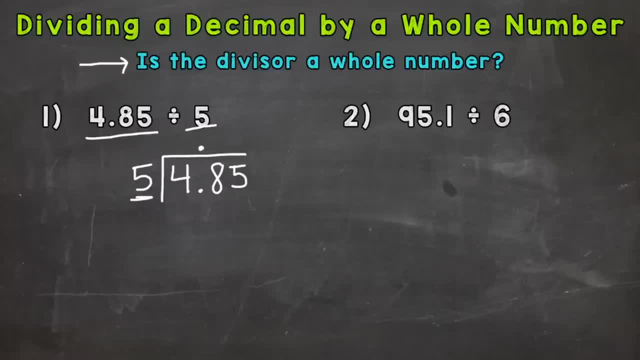 you do that. you just go through the division steps like any other long division problem: Divide, multiply, subtract, bring down and repeat. So we can start with 4 divided by 5. And we can't divide 4 by 5 and get a whole number. We can't pull any whole groups. 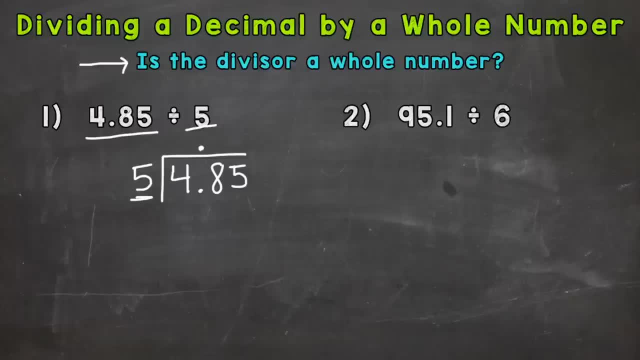 of 5 out of 4.. So we need to jump over to 48.. We need to include the 8 here, So we can put a 0 here if we want, because we can't do that. So 48 divided by 5. How many whole groups of 5 out of? 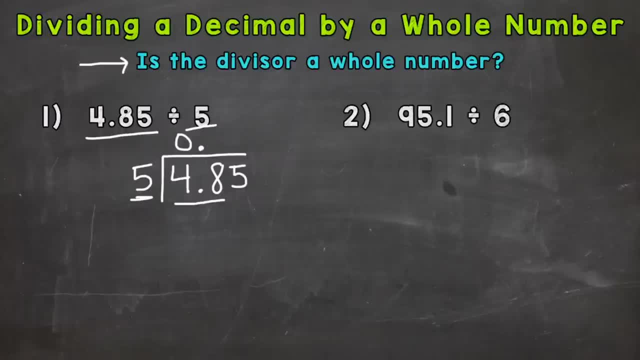 48?? Well, we know, 5 times 9 is 45. And that's as close as we can get. So 9 whole groups of 5 out of 48. Now we multiply 9 times 5, 45.. 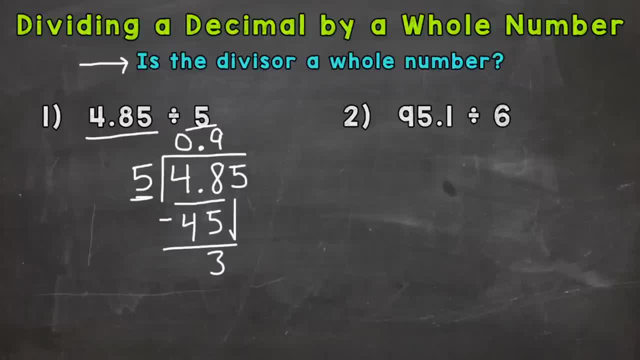 Subtract, we get 3.. Bring down And we have 35 divided by 5.. So how many whole groups of 5 out of 35?? Well, 7.. And we hit 35, exactly. So 7 times 5, 35.. Subtract, and we get 0.. So our answer is: 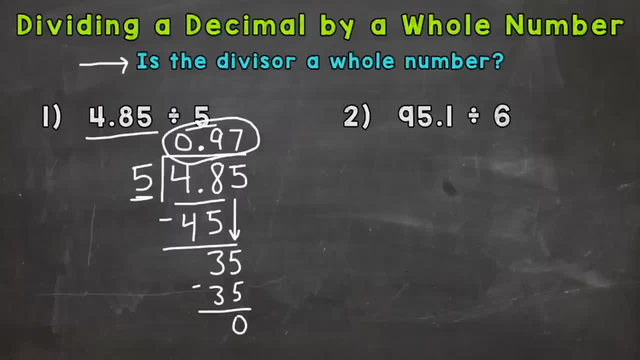 97 hundredths. Now number 2 is going to be a little bit different than number 1.. So please stick around for number 2.. And you'll see why towards the end of the problem. But the setup is the same. So 95 and 1 tenth is 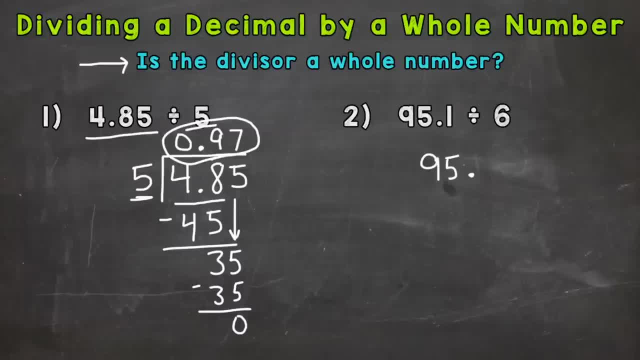 our dividend. It goes underneath our division bar. It's the number being split up or divided. 6 is our divisor, So it goes on the outside here. Now. we always ask ourselves this question, Although we know the answer to it in this video. you will get to a point where you have mixed up. 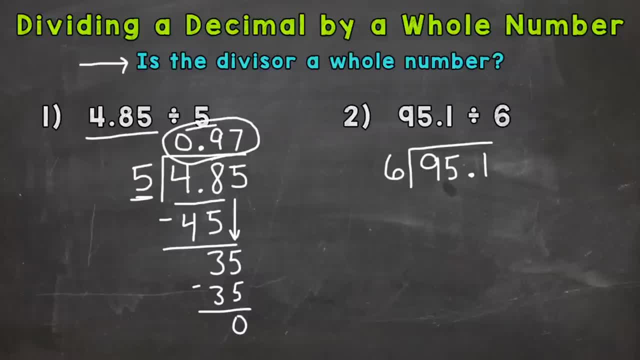 problems. So 95 and 1 tenth divided by 6.. Is the divisor a whole number? Yes, So we can bring our decimal straight up. It's going to be straight up within our answer there. Now we start our division process. So 9 divided. 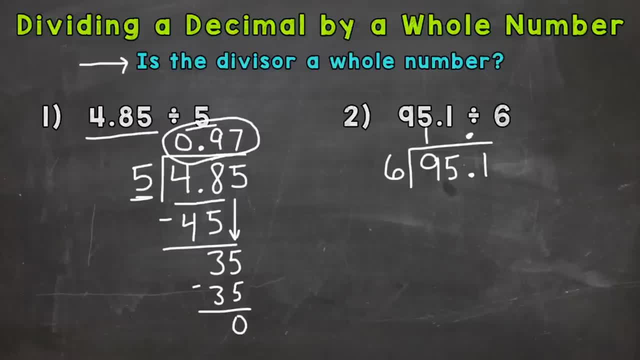 by 6.. How many whole groups of 6 out of 9?? Well, 1.. 1 times 6 is 6.. Subtract we get 3.. Bring down our 5.. Now we have 35 divided by 6.. So how many whole groups of 6?? 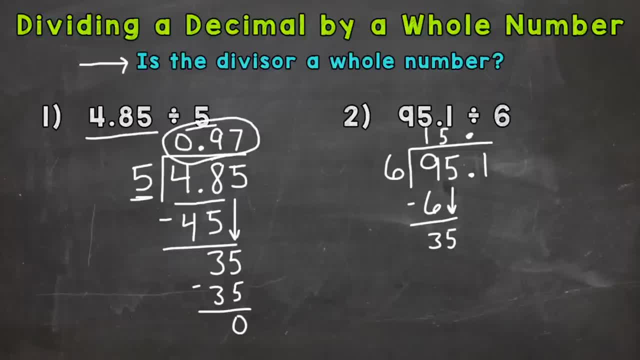 Well, 5. That gets us to 30. So 5 times 6 is 30.. Subtract, we get 5. And bring down this 1. So now we have 51 divided by 6. How many whole groups of 6 out of 51?? Well, 8. That gets us to 48. So 8 times 6. 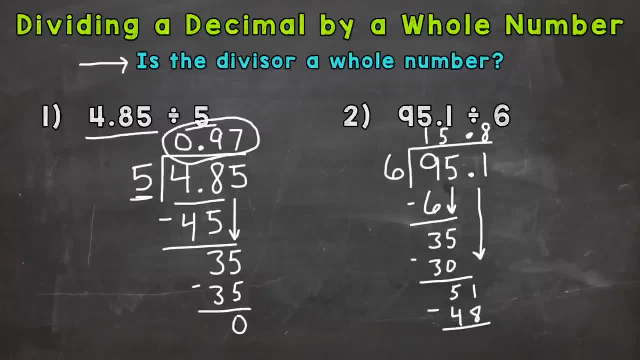 is 48. Subtract and we get 3. Now we went all the way over and we don't have anything else to bring down. So this is something we cannot do. We do not put 15 and 8 tenths remainder 3. Because 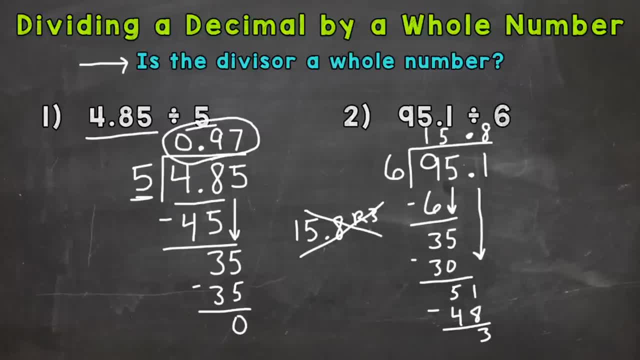 when we're working with decimals. any decimal within your answer is the remainder. So we are putting our remainder in decimal form, So we can't put a whole number there, a remainder 3.. So we need something to bring down without changing the value of our dividend there. 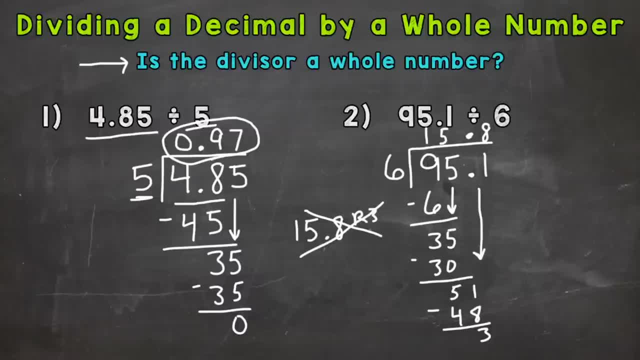 95. And 1 tenth. So what we can do, we can add a 0 here, Place a 0 on the end of 95 and 1 tenth, Because placing 0s at the end of a decimal does not change the value. That's an equivalent decimal. 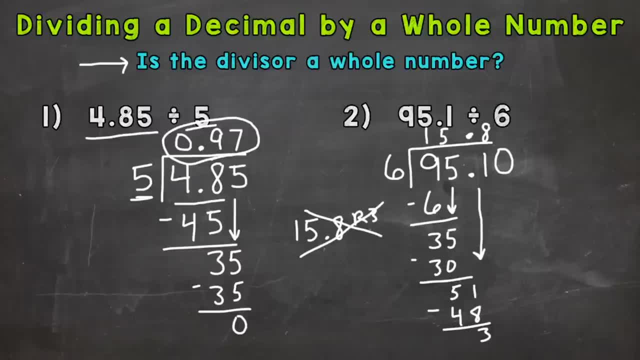 We did not change the problem at all. So now we have something to bring down. So if you ever get stuck there, place a 0 on the end and bring that down. Now we have 30 divided by 6.. Well, we can. 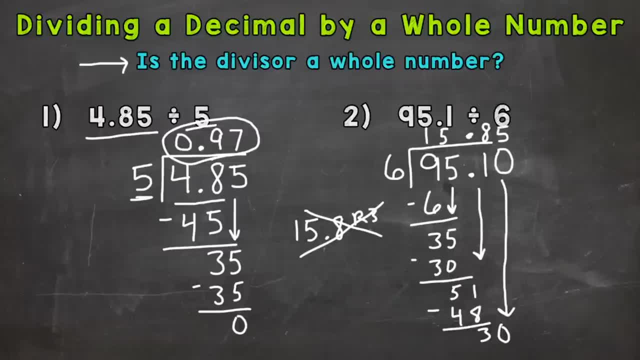 pull 5 whole 6s So we have 5 whole 6s. So now we have 5 whole 6s. So now we have 5 whole 6s. So now we have 5 whole 6s out of 30. So 5 here 5 times 6 is 30.. I'm running out of room here And 30. 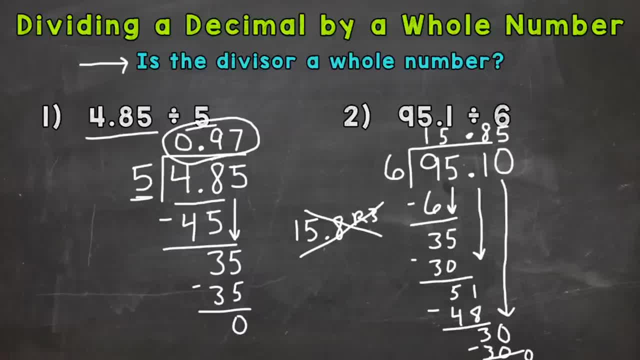 minus 30 gives us that 0. So we ended with a clean cut 0 there And our answer is 15 and 85 hundredths. Now some problems require you to place multiple 0s on the end And some decimal. 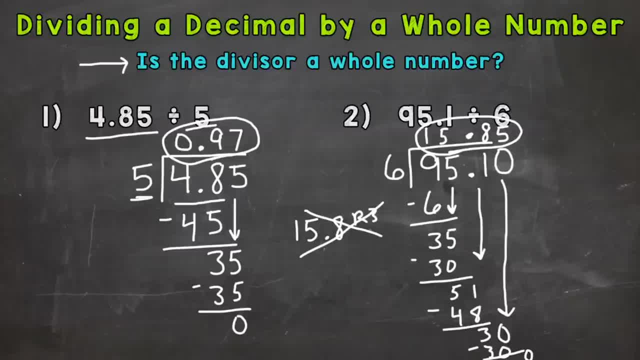 division problems never end. So there's a whole bunch of situations out there. But as long as you know that you can place a 0 on the end, you can place a 0 on the end. So you can place a 0 on the. 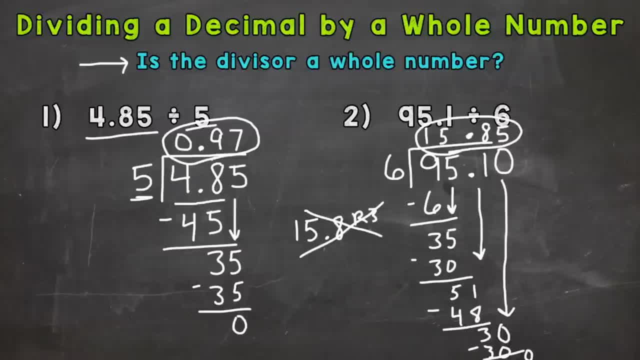 end. Bring that down in order to continue the problem until you get a clean cut 0 there, So 15 and 85 hundredths again is the answer to number 2 there, And that is how you divide a decimal by a whole number. Key points here: Check to see if your divisor is a whole number. If so, bring that. 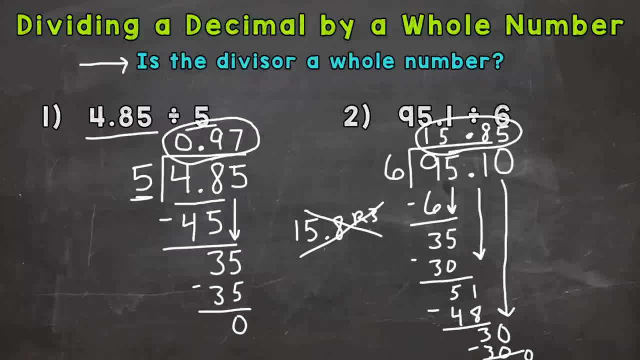 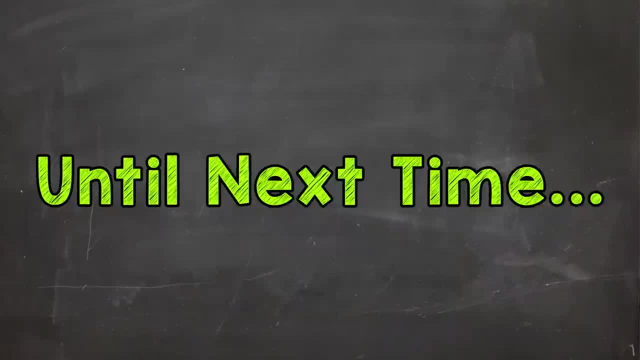 decimal straight up and go through your division process. I hope that helped. Thanks so much for watching. Until next time, peace you. 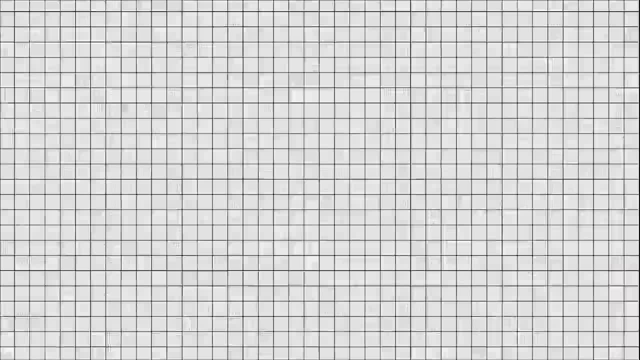 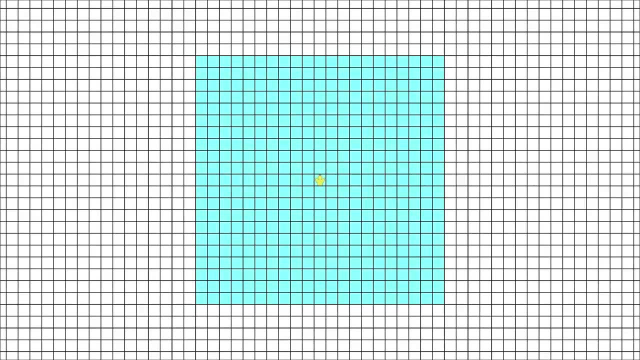 Shall, we play a game. You're an angel on an infinite grid. Each turn you can jump up to K spaces away. Let's say K is 10 for this example, meaning that you can jump to anywhere within this boundary, But your arch-nemesis, the devil, is watching.